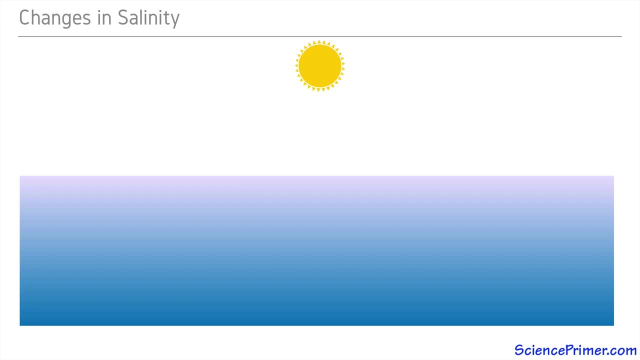 cooler, denser water. If this was all that was going on, then no mixing would happen. but there is another factor that influences density of water: Salinity. Ocean salinity, that is, the concentration of salt in the water, is fairly constant over 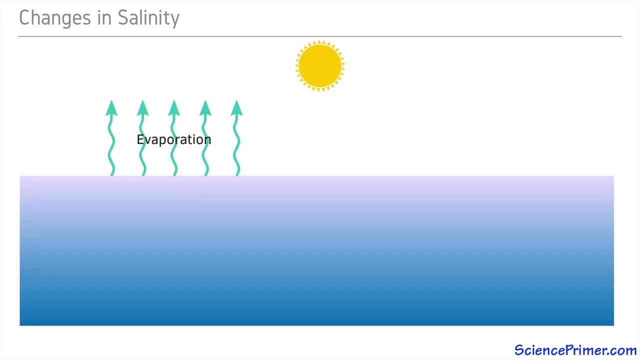 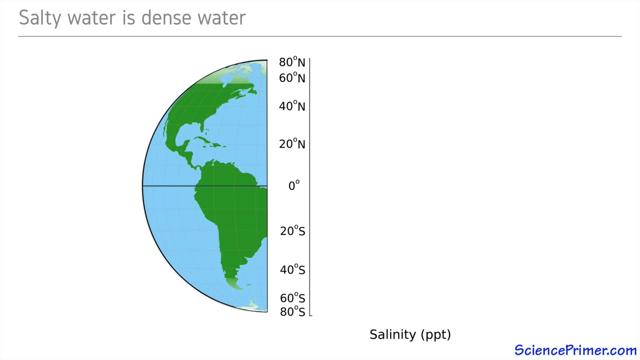 space and time, but small variations do occur due to patterns in evaporation and precipitation, which cause surface salinity to vary between regions of high and low rainfall. The zone of precipitation associated with the low pressure system around the equator causes lower salinities. 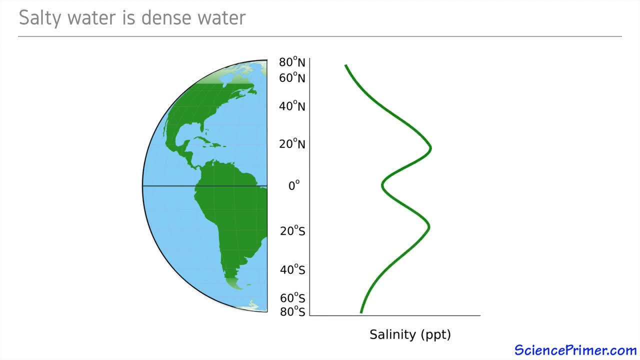 near the equator. Salinity then increases through the mid-latitudes due to evaporation, where the lower portion of the Hadley cell, the lower portion of the ocean, is the salinity. Salinity then moves dry air towards the equator. Salinity then decreases again towards the poles, where there 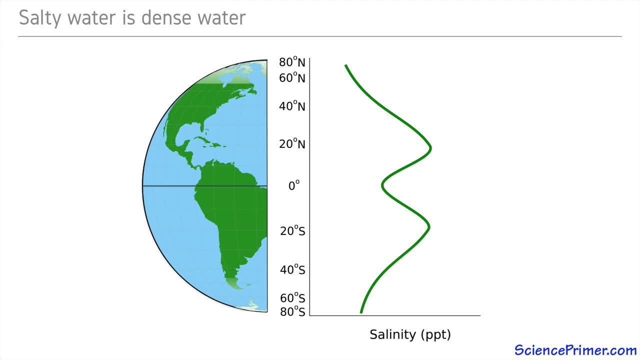 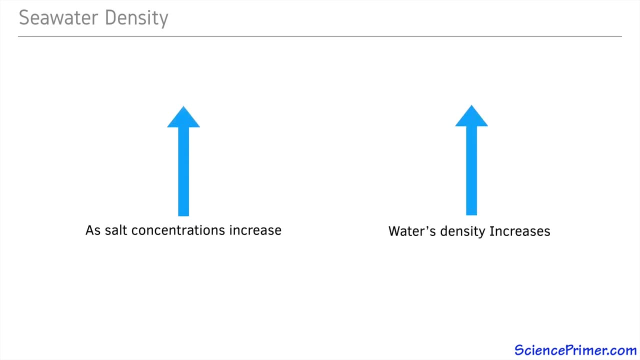 is an increase in precipitation associated with the low pressure region stratification at low latitudes. The transition region between the top layer of warm water and cooler water below is called the thermocline. As we move poleward and the amount of solar energy reaching the surface of the earth goes, 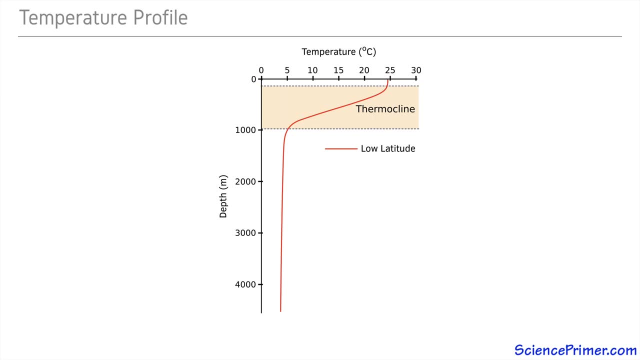 down, the thermocline breaks down and temperature from top to bottom in the ocean evens out. Close to the poles there is little or no temperature difference from surface to bottom. The evening out of density creates a situation where mixing from top to bottom is possible. but simple mixing is not sufficient to 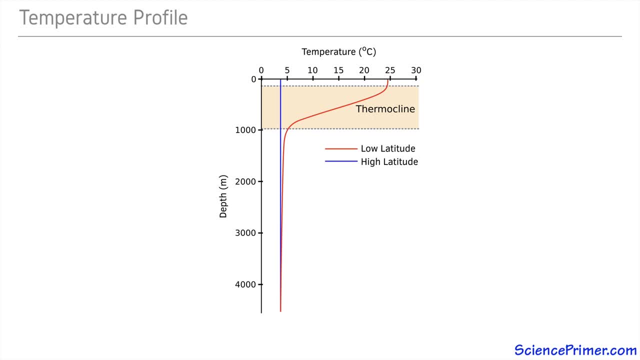 drive density-driven circulation, in which dense water sinks to the bottom near the poles and then flows equatorward under less dense water. In order to get density-driven circulation from high to low latitudes, changes in both temperature and salinity are required. The way this occurs near the poles on earth is: 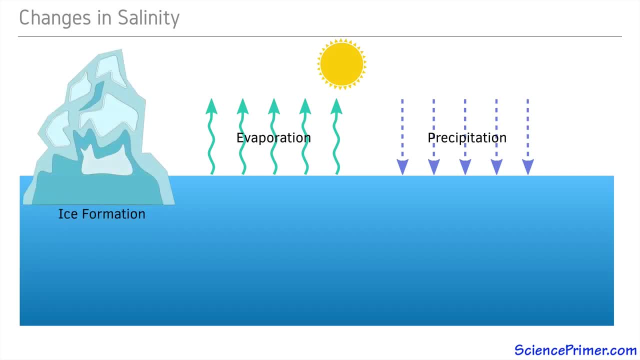 through the process of ice formation because, as saltwater freezes to form ice, the ice crystals exclude the salt, increasing the salinity of the water left behind. So in regions near the poles, where significant ice formation occurs, the temperature changes from high to low and the temperature changes from high to low. So in regions near the poles, where significant ice formation occurs, the